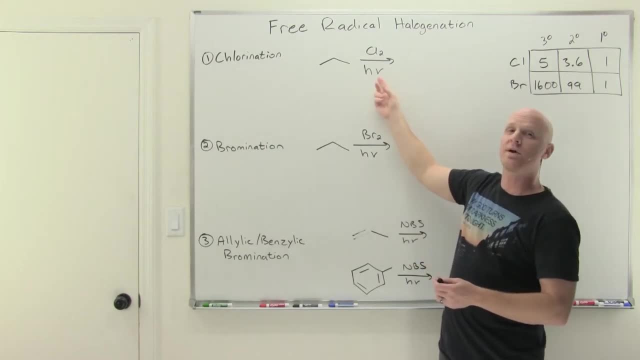 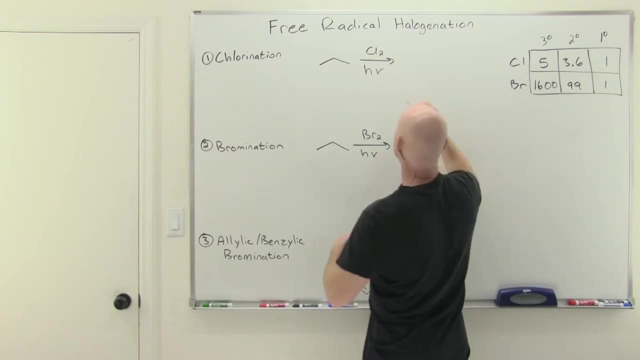 common one you'll see, and it's probably the one I'll use pretty ubiquitously here. but you could see heat or an epoxide here- I'm sorry, heat or a peroxide here- pretty commonly as well. So if we look at what's really going on here, we've got a couple of different products here and you look 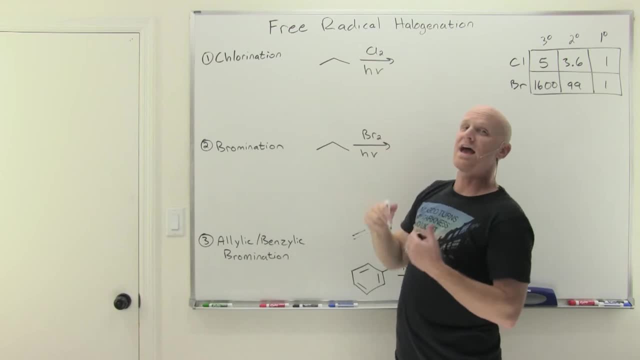 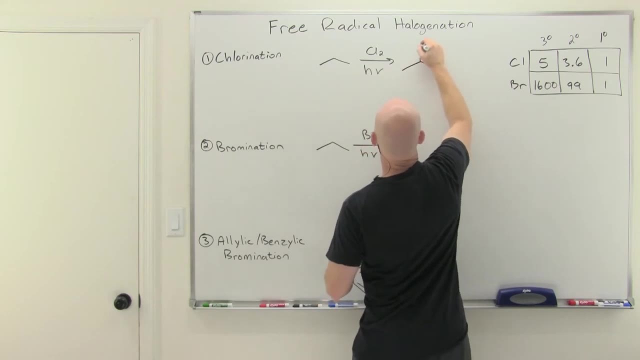 at the different hydrogens on here and there are two hydrogen environments here And if we replace any single hydrogen with a chlorine, that would be called a monochlorination reaction here And it leads us to two products here. That's these two here. I can replace either one of the two. 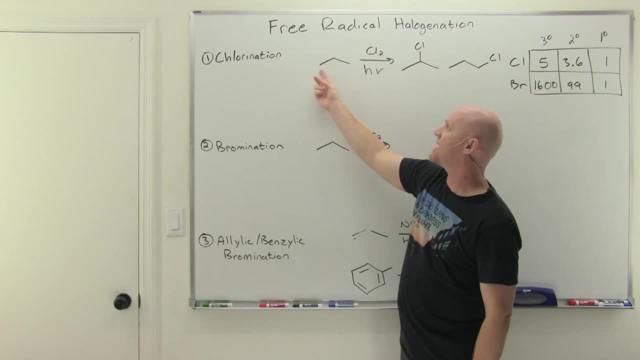 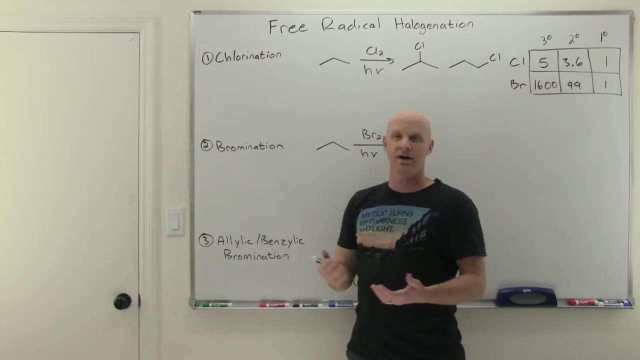 hydrogens on that carbon to get this product, or any one of the six hydrogens on these two carbons, since they're equivalent, to get this product. It didn't matter if I put the chlorine on the right-hand side or the left-hand side, It's the same thing either way. one chloropropane. 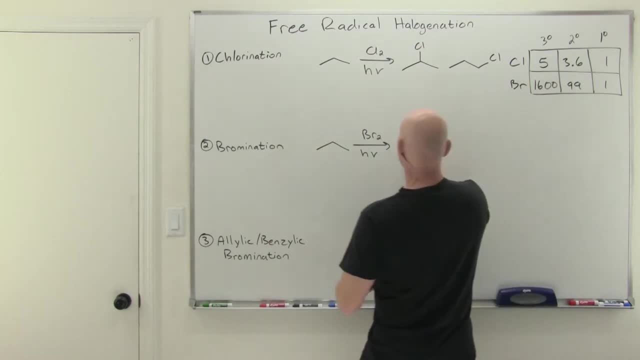 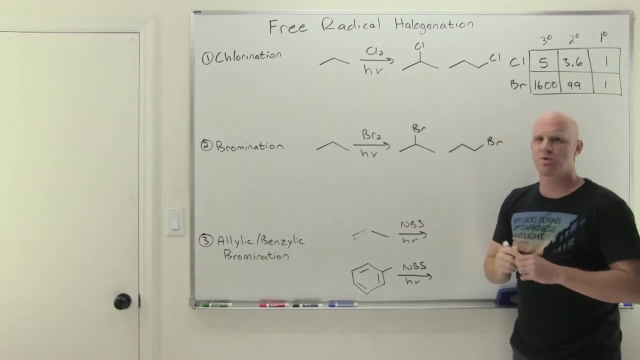 Cool Bromination works exactly the same way, but the result's going to be a little bit different, as we'll see. You can't tell the difference just yet, but what you'll find out is that the bromination reaction is much more selective. So the chlorination it turns out. you look at all the possible products. 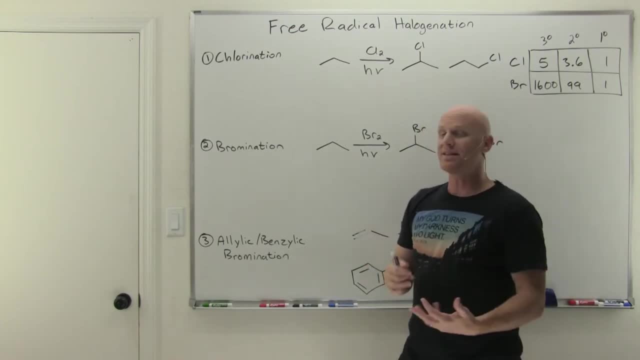 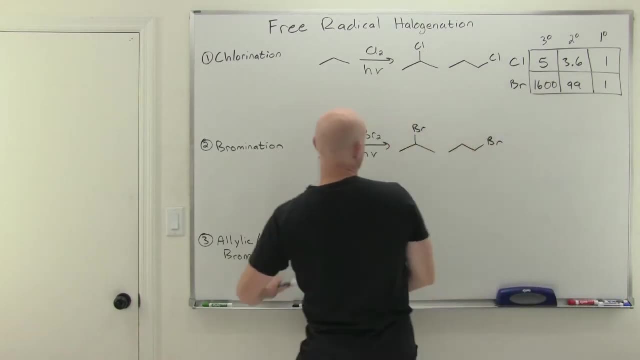 and you can expect to get a bunch of all of them, So at least a fair amount of all of them. But with bromination, if you look at your different products, it's a much more selective reaction And if you kind of take a look here we've got the bromination on a secondary carbon here. 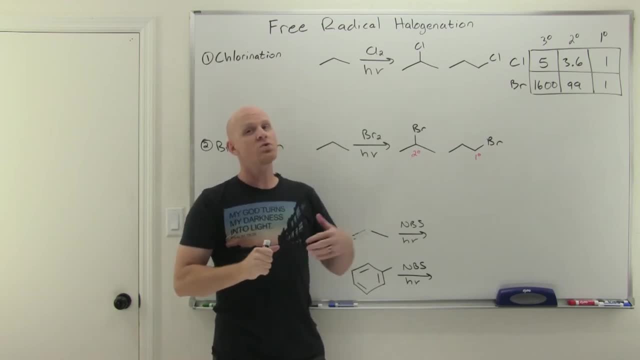 and on a primary carbon here, And what you'll find out is that you are overwhelmingly going to get just this product on the left. I'm not saying you'll get this product on the left. I'm not saying you'll get this product on the left. 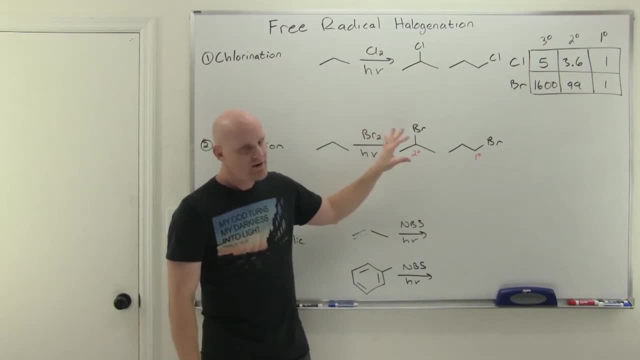 You're going to get zero of the product on the right, but you're not going to get very much. So bromination is a nice reaction in that respect. if you're trying to selectively get a single product, Much better, Whereas again, with chlorination, way less selective. 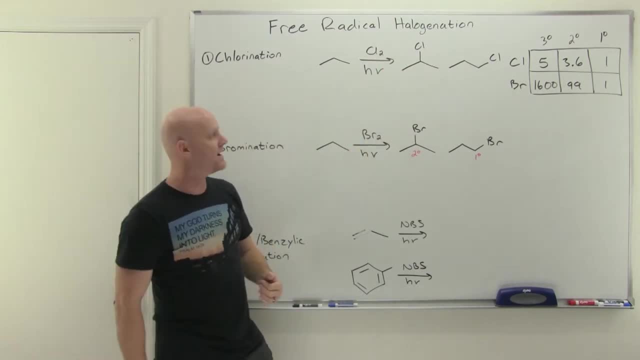 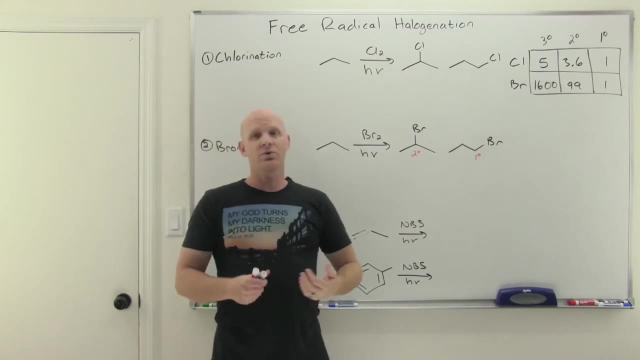 as we'll find out And we'll talk about it in the mechanism- why exactly it's not so selective, but bromination is. But you can expect to get a mixture of products And we'll talk a little bit about how you come out with predicting relative ratios of products and stuff like that. That's. 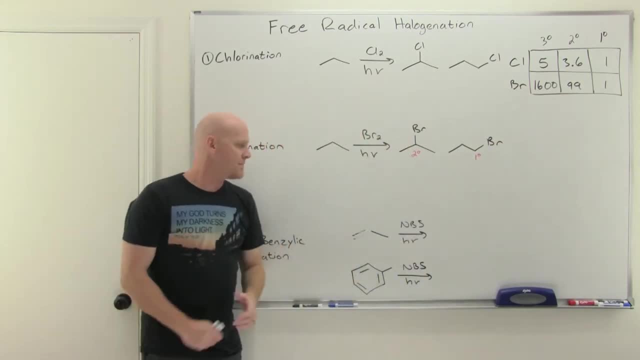 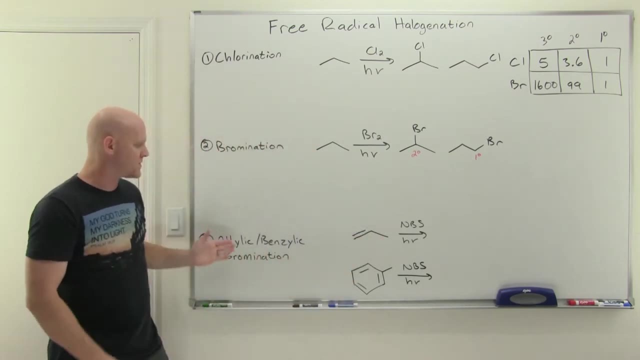 what this lovely table will be for when we get there in a second. But before we get there I do want to talk one second, And it looks like I pressed up against the board here, So let's get that back in place. But I want to talk about what's called allylic or benzylic bromination. 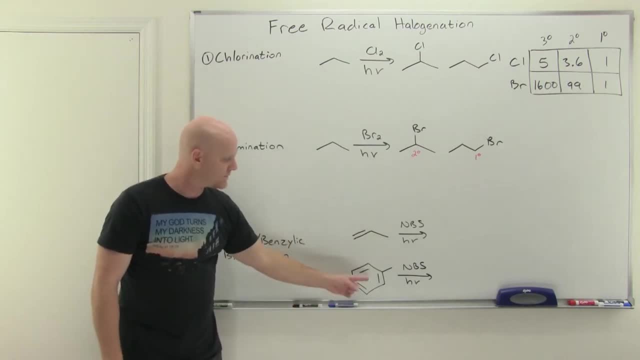 And if you've got an alkene and you identify your allylic carbon, or if you've got a benzene ring and you identify your benzylic carbon. So reminder that allylic means one carbon away from an alkene, or benzylic means one carbon away from a benzene, And specifically it turns out you could try to. 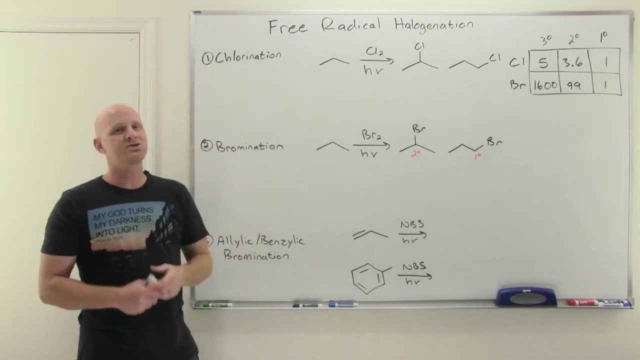 use bromine here, And it turns out you're going to end up getting a mixture of products, So Br2 can either be an alkene or benzene in other reactions besides the one of interest here, And so we end up using a little bit different reagent called NBS, which stands for N-bromo-6-cinnamide. We'll have 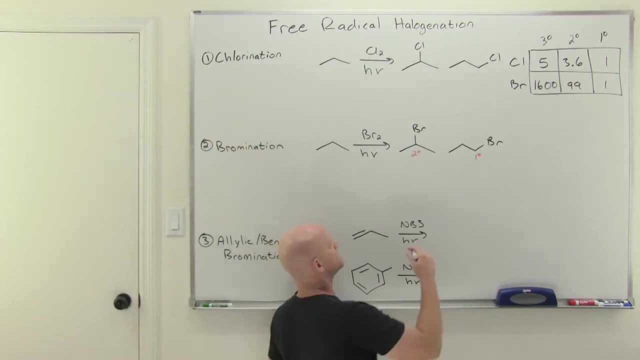 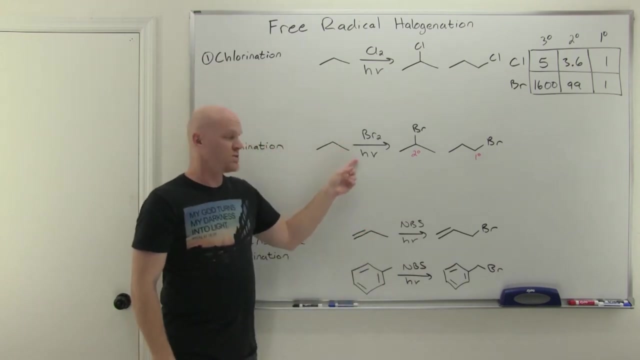 a whole lesson on this in the third lesson in this chapter, But I just want to allude to it here. And so if your goal is to specifically brominate in the allylic or benzylic position, this is the reagent of choice. Cool, It turns out, just using Br2 and light would not accomplish the task very. 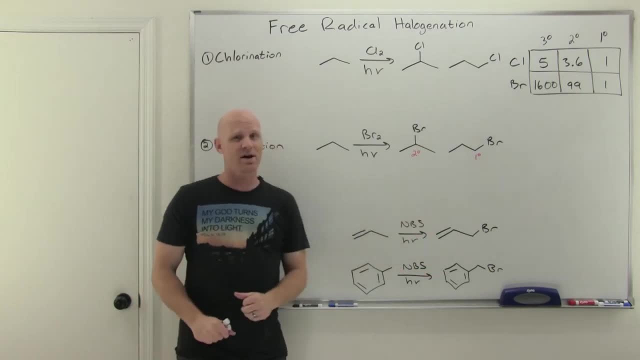 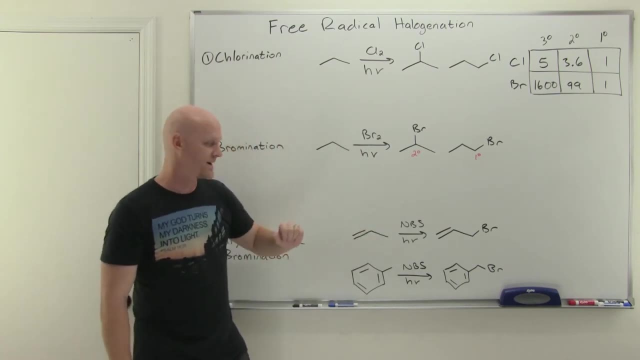 well, You'd get a bunch of side effects. You'd get a bunch of side effects. You'd get a bunch of side products in addition to your desired product here. So if your goal is to brominate either allylic or benzylic, don't use Br2.. So use NBS instead. Like I said, we'll come back to talk a. 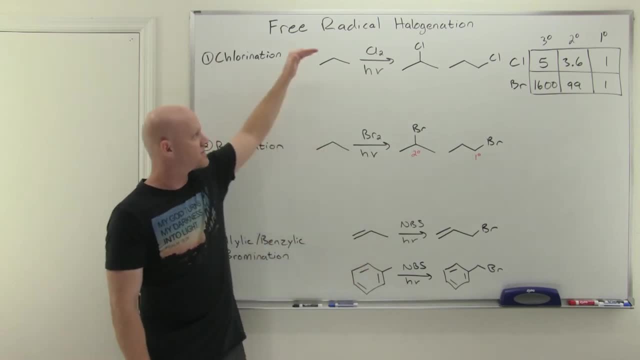 little more about NBS, So I just want to allude to it here and just kind of show the three different free radical reactions, But we'll spend a whole extra lesson on this one later in the chapter. All right, So if we take a look at chlorination and bromination yet again? so we said that. 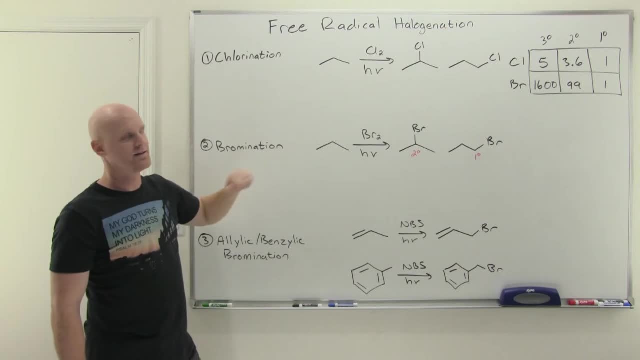 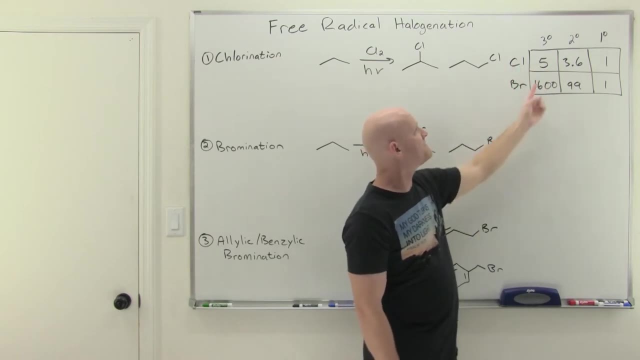 chlorination is not so selective, but bromination is highly selective And in this case we can get the idea based on some ratios here. So with chlorination it turns out you are five times more likely to replace a tertiary hydrogen than a primary hydrogen And you are 3.6 times more 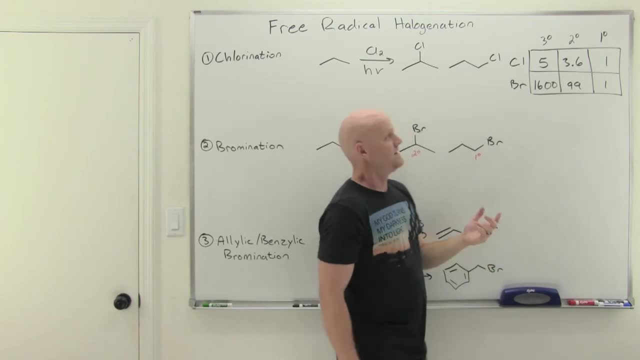 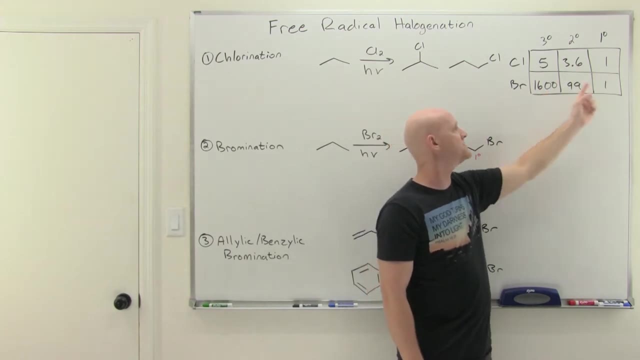 likely to replace a secondary hydrogen with a primary hydrogen. So that's kind of the way those ratios work Well. with bromination, you are 1,600 times more likely to replace a tertiary hydrogen than a primary hydrogen and 99 times more likely to replace a secondary hydrogen. 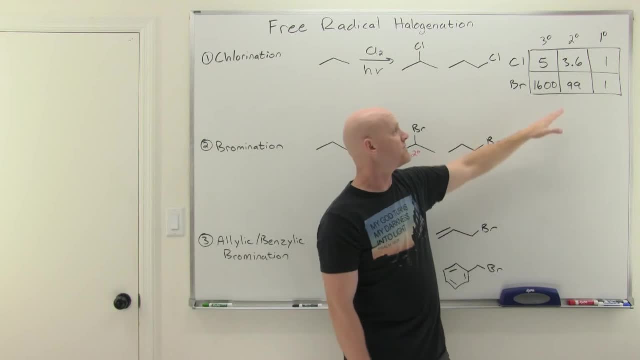 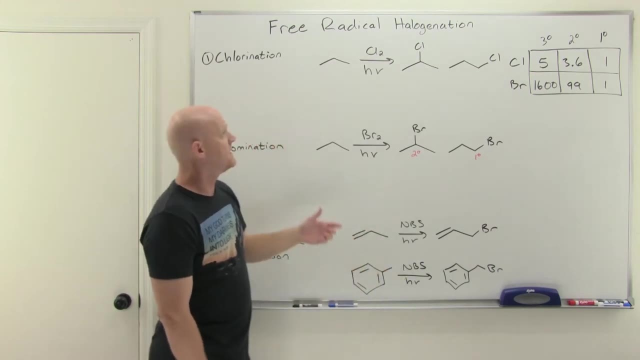 with a uh than a primary hydrogen. So all of a sudden, this is a reflection of that selectivity where it prefers replacing a hydra on the most substituted carbon possible, overwhelmingly so. So if we take a look at what's going on here, so if I I told you that, uh, you. 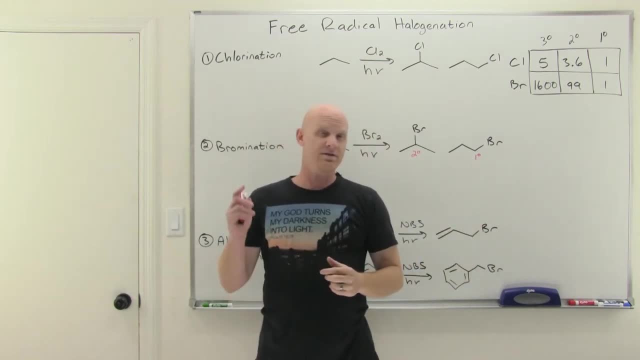 know I was 10 times more likely to win the lottery than you today. So then you might tell me: well, Chad, go play the lottery. So, and if I said well, then who's more likely to win the lottery? 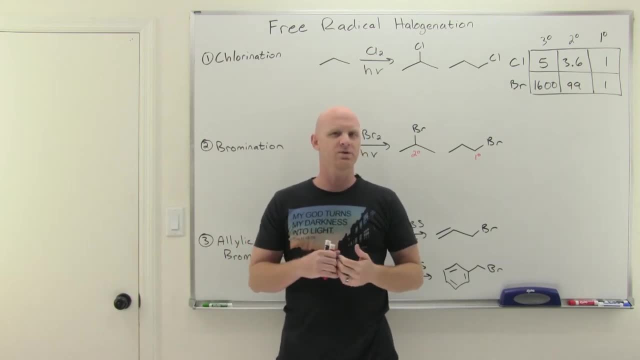 me or you? Well, you actually can't answer that question. You might be like: well, you just told me you're 10 times more likely. Well, that's assuming we buy the same number of tickets- 1,000 tickets. Well, even then, you know, ticket for ticket, I'm 10 times more likely to win You. 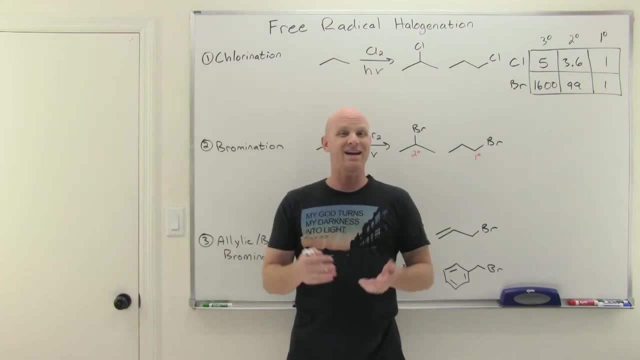 bought a thousand times more tickets and you factor both things in and now you're a hundred times actually more likely to win the lottery today. So I'm 10 times more. you know luckier if we will, but you bought a thousand times as many tickets, which overwhelmingly makes up for. 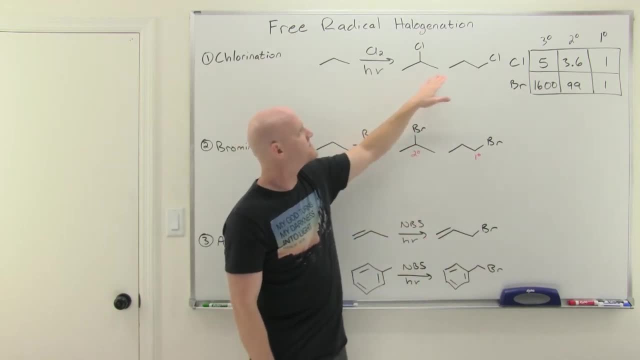 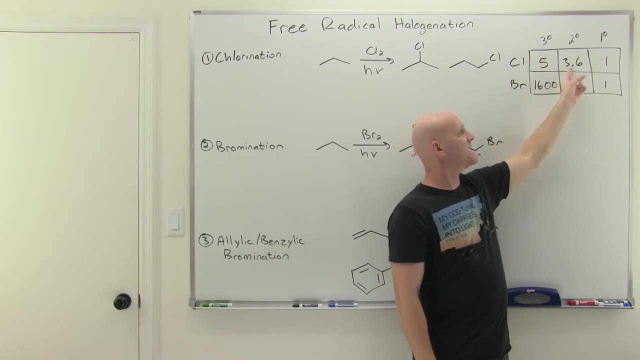 that And then some. well, the same kind of thing here when you're when you're looking at your different chlorination bromination products. if you want to predict relative amounts of these products, you've got to factor in. you know how much more likely you are to. 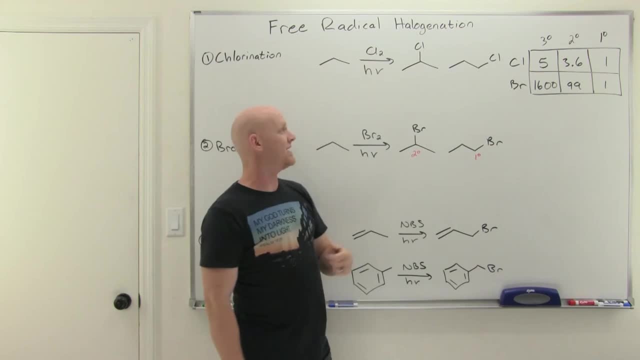 substitute at one position versus another, but then also, how many chances do you have? So, to get this product right here, I've got to replace either one of the two hydrons attached to this carbon, And so they're not just one chance, there's two chances. So, and it's on. 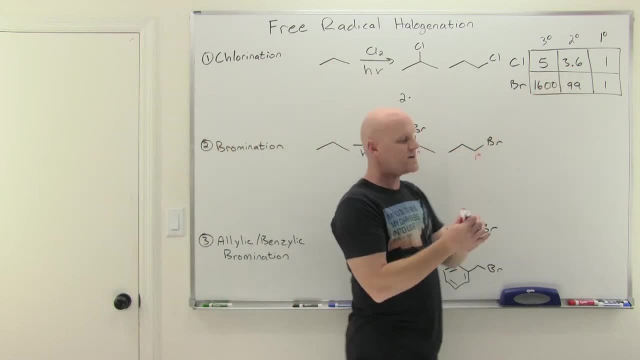 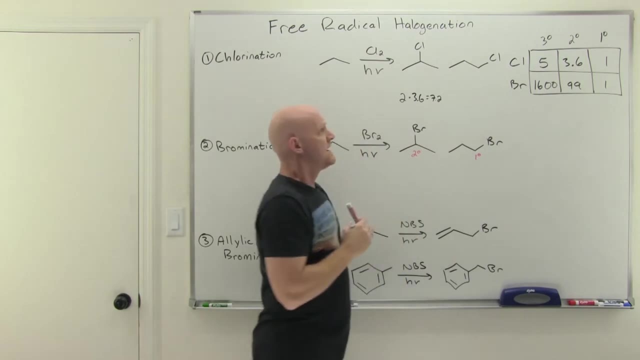 a secondary carbon there, And so the likelihood here is 3.6,, if you will, And so I'm going to multiply this by 3.6, that's going to get a 7.2.. And if we look at you know the likelihood of. 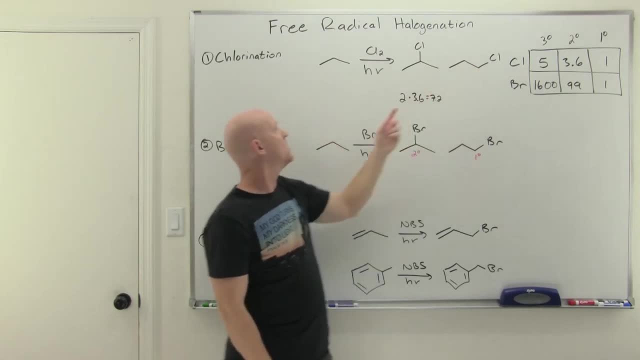 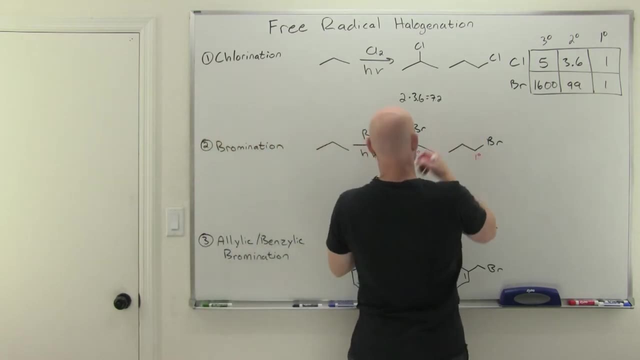 replacing one of the hydrons to get this chlorination product. well, again, there's any one of these six hydrons, any of the three on this carbon, or any of the three hydrons on this carbon, And so we've got six chances now for this one, And in this case, though- but it's on a primary- 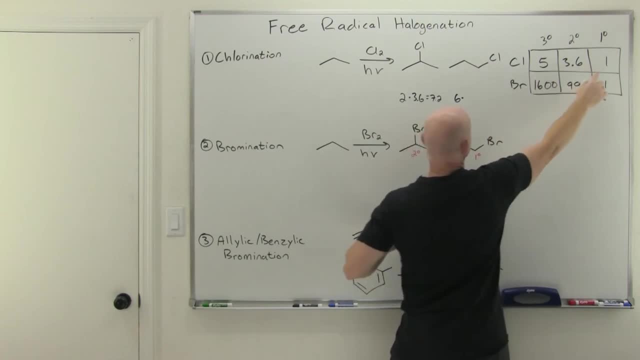 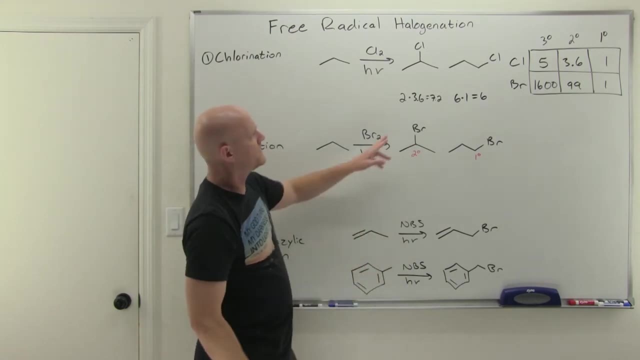 carbon. these are both primary carbons, and that's just got a likelihood, if you will, of one And six times one is six, And so this can kind of give us some relative amounts here, And so what we'll do is we'll take and add these together to get a total of 13.2.. 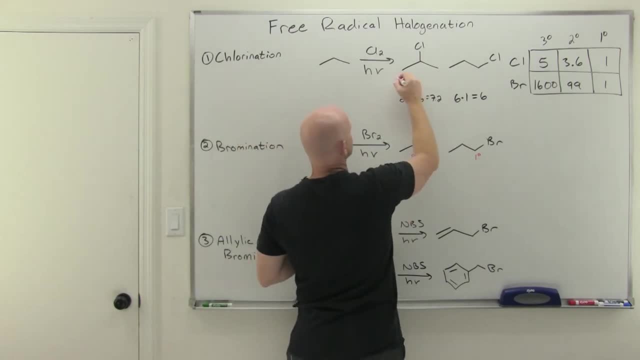 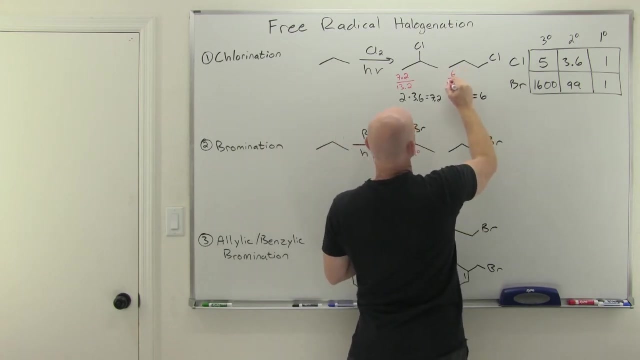 And so the likelihood here of getting this particular product is 7.2 out of a total of 13.2, just adding up the sums of all the products that are possible here. All right, And then the likelihood of getting this product here is going to be six out of 13.2.. And then times 100, if you. 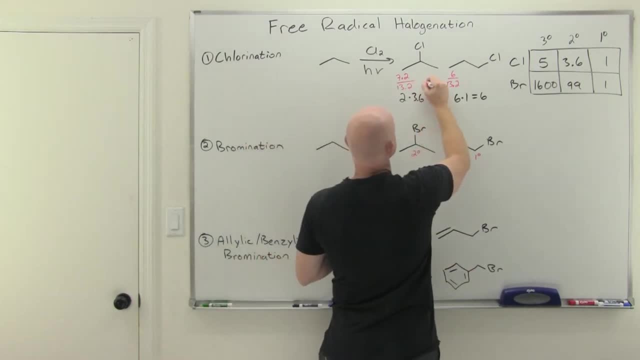 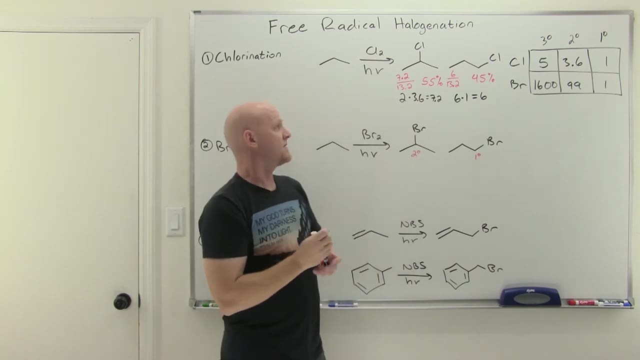 want to turn it into a percentage, And in this case, that's going to come out here, in this case, to somewhere right around 55% for this product and 45%, And so you might've been like, Whoa, you're 3.6 times more likely to get the secondary product. Well, 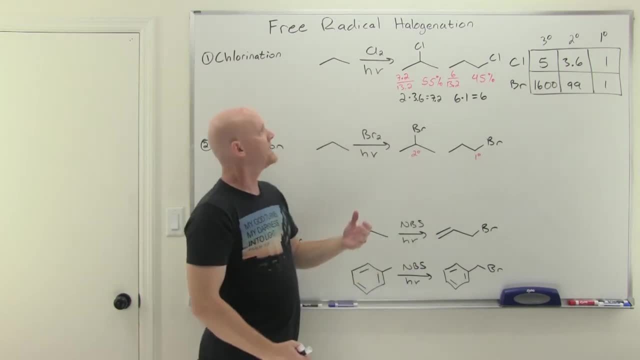 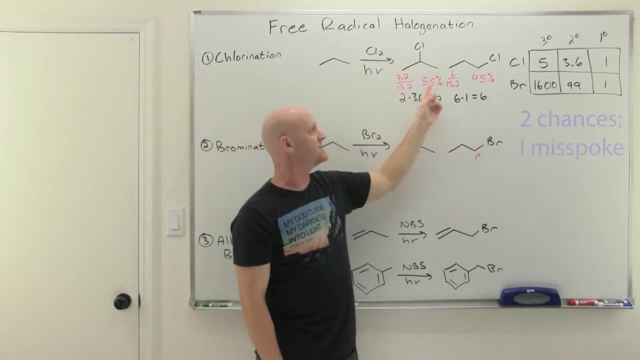 again, as long as you've got the equal number of chances. but I got six chances to form this product. I've only got one chance to form this product And so, as a result, they actually come out fairly even So, 55% versus 45%, but the first one would be the major product, but it's close. 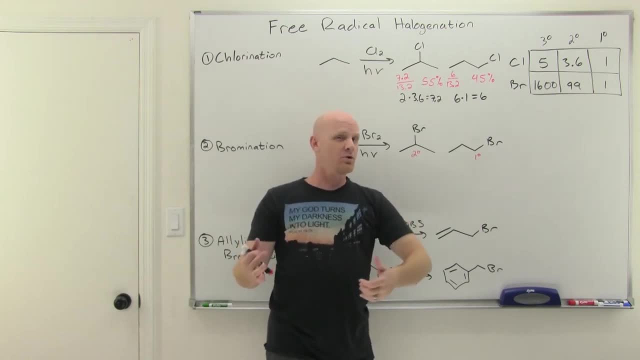 And so, like we said, chlorination is not very selective. If you've got multiple products, you can form. you're going to form some of all of them, All right. But if we take a look at the same kind of calculation with bromination, you're going to see that you're going to see that you're. 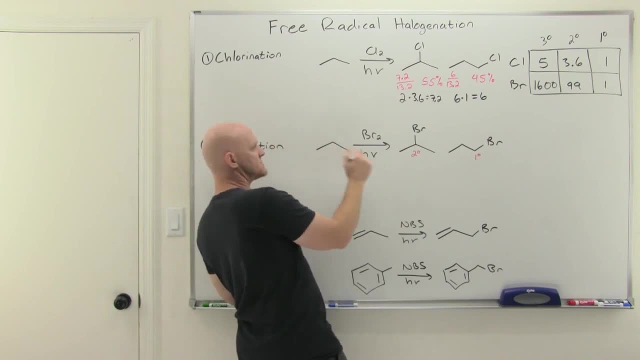 going to get this product. So this is a carbonation And once again we've only got two chances to form this product. One of two hydrogens we can replace right here, So, but for a secondary carbon it's 99 is the relative likelihood there. So six chances, six different hydrogens we could. 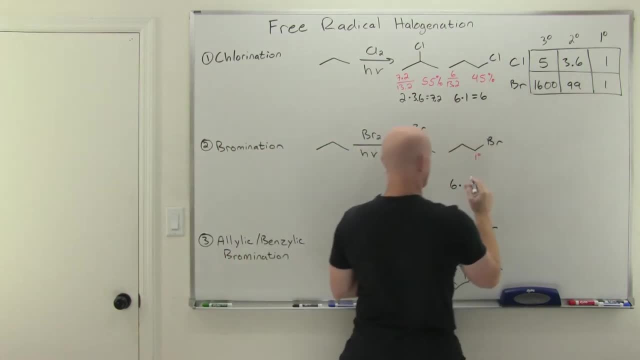 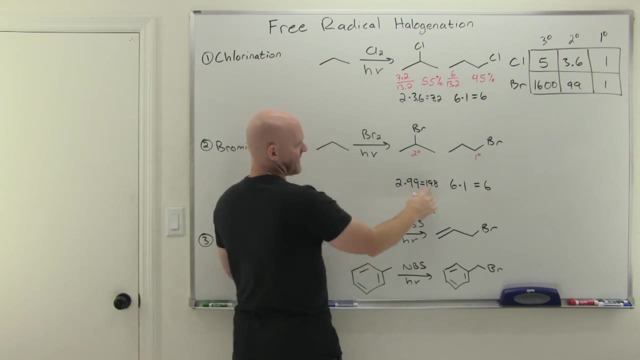 replace to form this product. And so we'll take six, but just times again, a relative likelihood of one and six times one is six, two times 99 is 198.. And so in this case, if you add 198 and six, 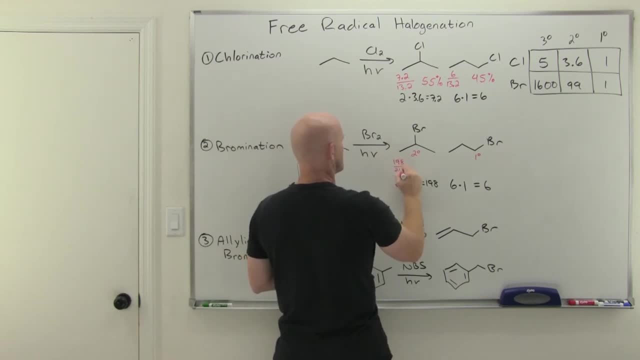 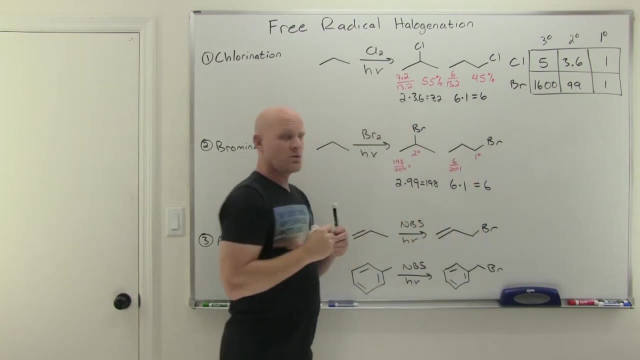 you're going to get 204. And so we've got a likelihood of 198 out of 204 for this one. and then again, times 100 and this one only six out of 204. so, and if you work this out and multiply by 100, you're going to get this one comes out to 97. 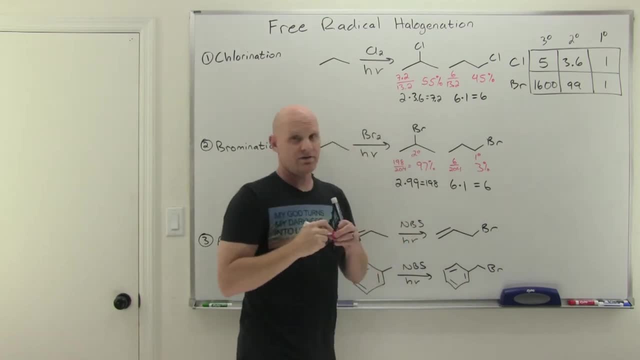 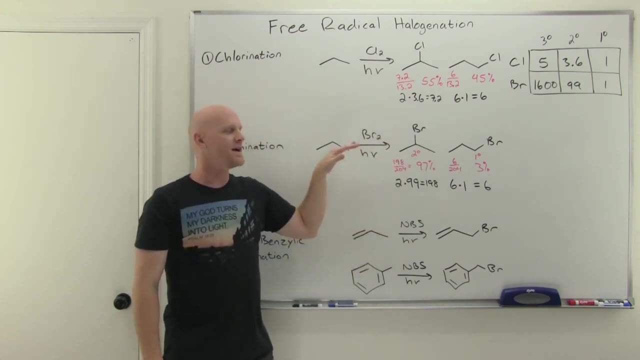 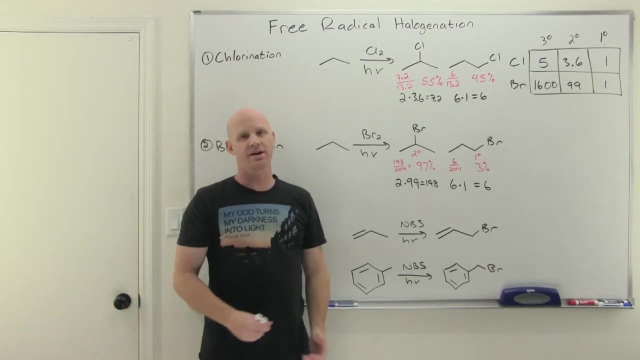 and this one three percent and notice, if you by all means get a chance to replace a tertiary hydrin, it goes up even higher to 1600, and so overwhelmingly you can get. you know, uh, one major product in bromination. oftentimes when you've got one substitution that's much more favored over any. 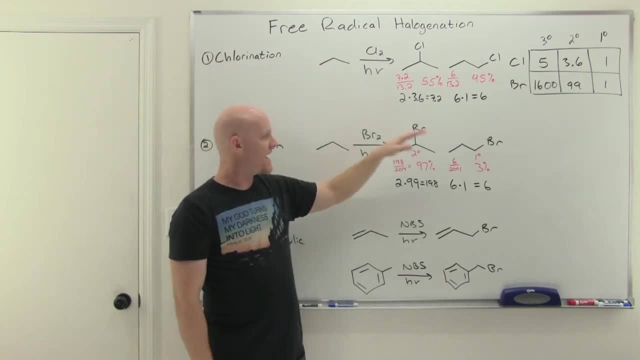 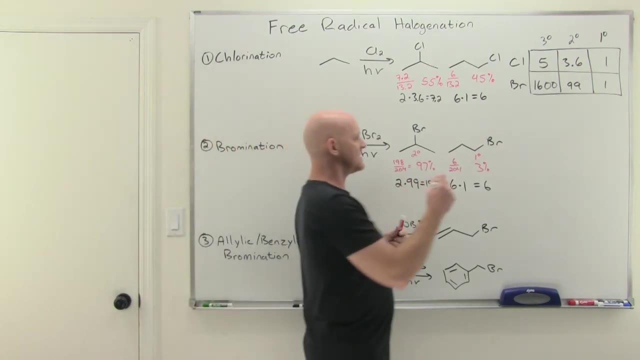 other. so if you're doing synthesis problems, we'll find out that we vastly prefer bromination much of the time, just because it is so selective and we can get just one product. now, if you've got, you know something like, say, cyclohexane. so in cyclohexane you've got 12 hydrins and they're 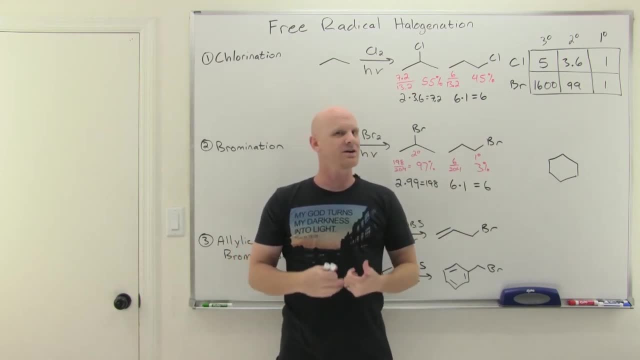 all equivalent. it doesn't matter which one you replace with a chlorine or a bromine, you're just going to get chlorocyclohexane or bromocyclohexane. so if you've got something like this, well then take your pick: chlorination, bromination, whatever. 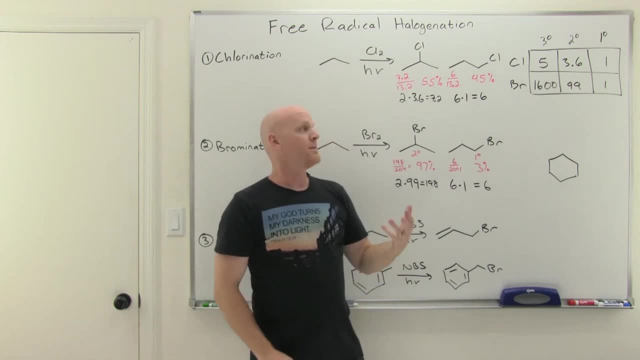 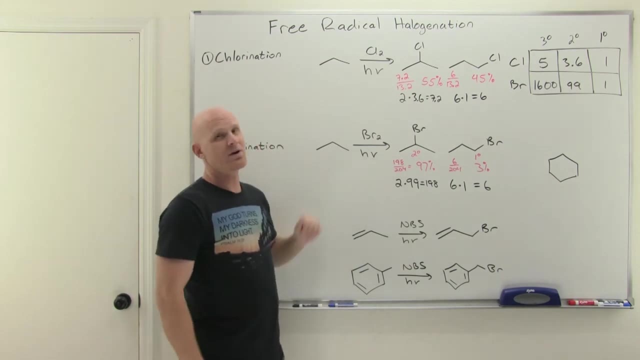 because you've only got one possible product, no matter what. but if it's something like propane here, you've got two possible products. if your goal is to get one single major product, then you're way better off using bromination. you'll find out that we use it way more often in synthesis. 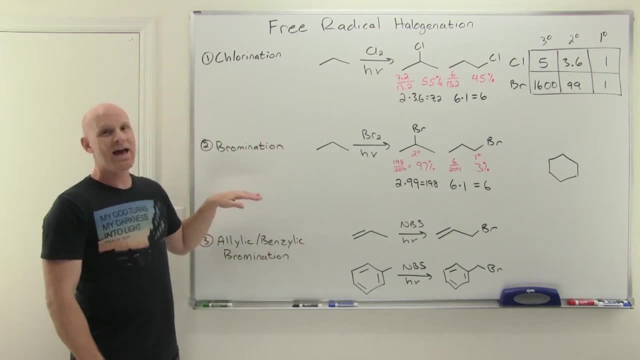 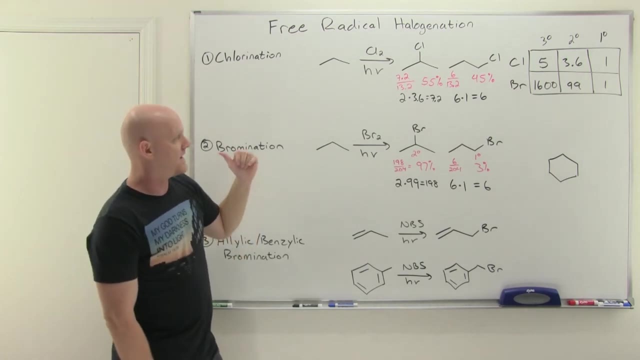 now one thing to note about nbs here. now it turns out nbs can do the same thing as as br2- i shouldn't really say cl3- but the same thing as br2. it's still selective so and it would still largely give you this major product right here. so 97 yield. 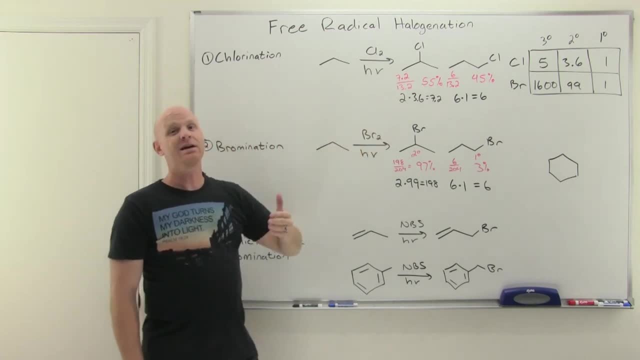 um. however, you probably wouldn't use it here if you were doing this in the lab. it would still work here, but it's more expensive as a reagent nbs than just plain old br2 and light, and so if you you were doing this in the lab, you just use br2 and light, so you specifically use nbs in the lab when. 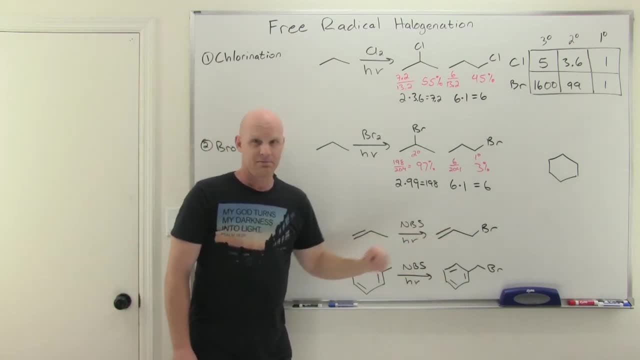 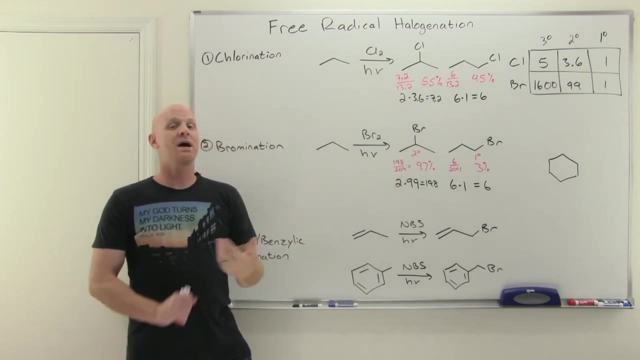 you're trying to again brominate allelically or benzylically. however, if you did it on paper, on something just like propane, it's not allelic or benzylic. it's still going to give you the same product as br2 and light. and on paper, that's beautiful. on a synthesis problem, that's beautiful. 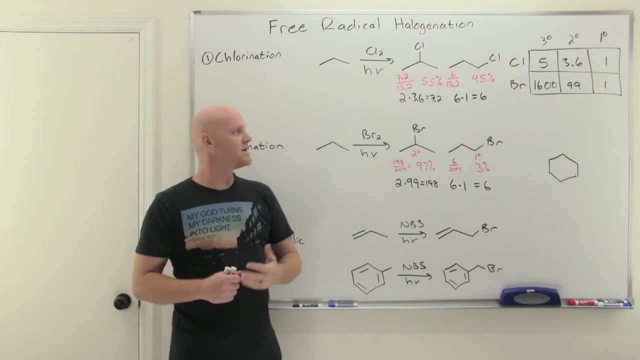 in the lab. it might be a little bit more expensive, but it's still going to give you the same product: waste of resources, a little more expensive and stuff. but on paper it is lovely and i just want to make sure you're aware of that because from a synthesis perspective, you know you got to make. 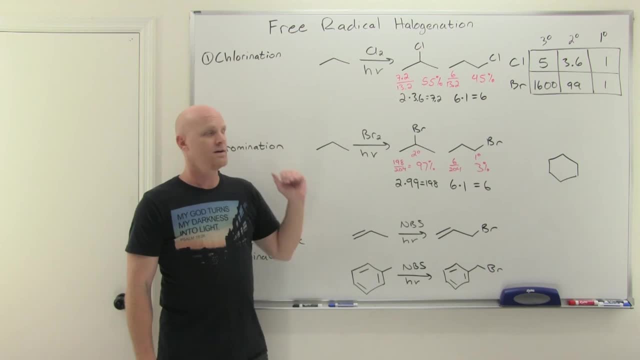 sure if, when it's allelic or benzylic that you have to use nbs, not br2. but if you're using something that's not allelic or benzylic, you can use nbs but you're probably more likely to use br2 in the lab. 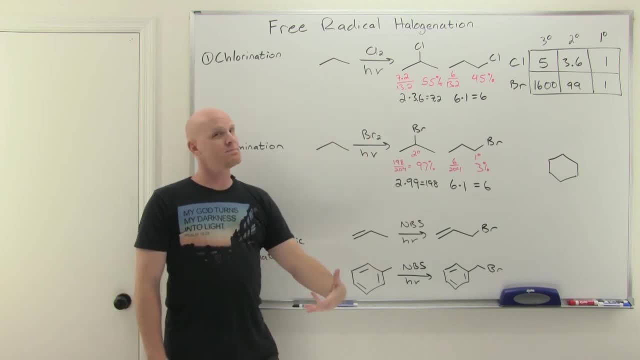 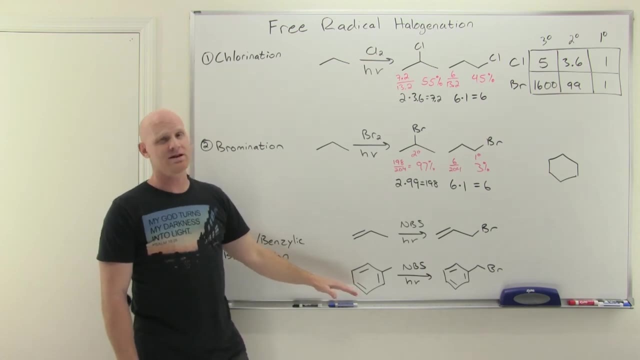 but which means if you're trying to brominate, you can always use nbs. but you got to be careful, you know, of when you use br2 versus nbs, because if it's allelic or benzylic, you have to use nbs, you don't have to use nbs. you don't have to use nbs, you don't have to use nbs. 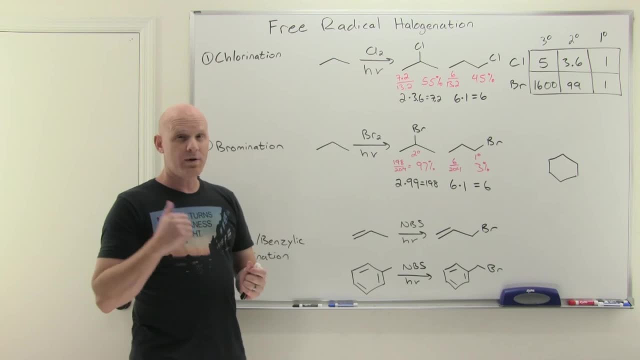 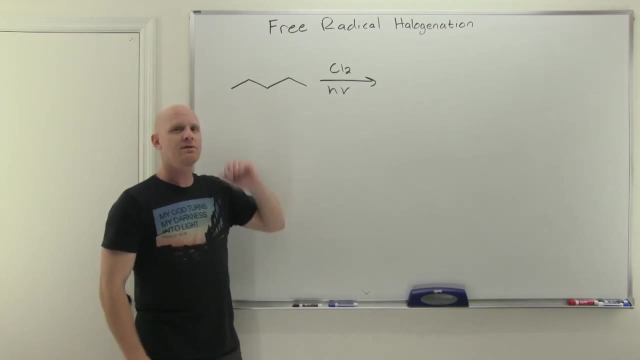 you want to make sure you're aware of that. let's take a look at one more type of question you might see in this context. so the other kind of question you might see regarding this is: it might give you a lovely reactant and then ask you the number of different, either monochlorination or monobromination. 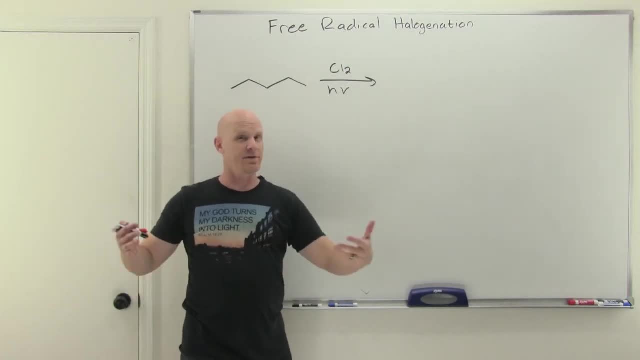 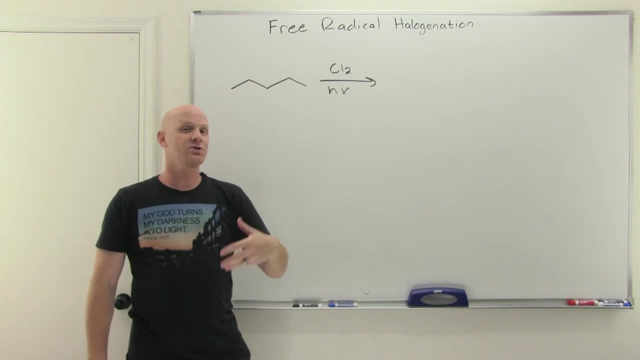 products and you're more likely to hear about monochlorination, because you will likely get all the products and a fair amount of each of them. so the question might be how many different monochlorination products are possible, and they might tell you to either include or exclude. 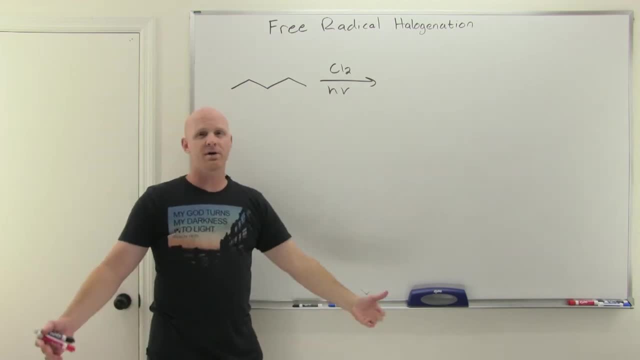 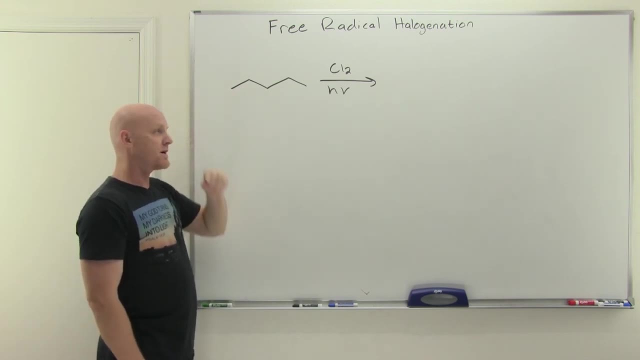 different stereoisomers and so in this case i'm going to have you include all the different possible stereoisomers, so you got to factor in if you're forming chiral centers in this stuff. so if you look at this, if you looked at this from like an nmr perspective, you might realize that 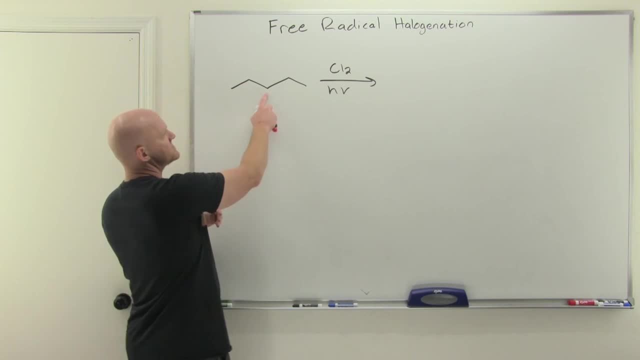 there's only three unique types of hydrons here. so these two hydrons are equivalent on this carbon. so the four hydrons on these two carbons are equivalent, and then the six hydrons on these two carbons are equivalent. so with three different types of hydrons we can substitute in three. 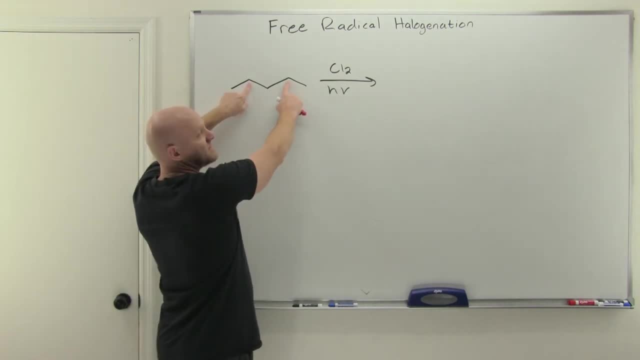 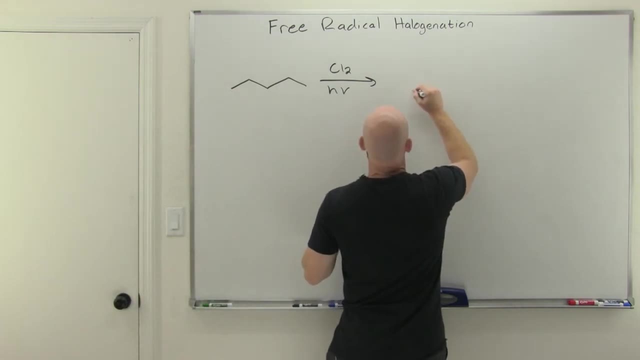 different places. i can substitute on the middle carbon. i can substitute on either one of these carbons, or i can substitute on either one of these carbons to get three fundamental different regio, ice, mers- let's draw those out. so again, i can substitute on the middle carbon. i can substitute. 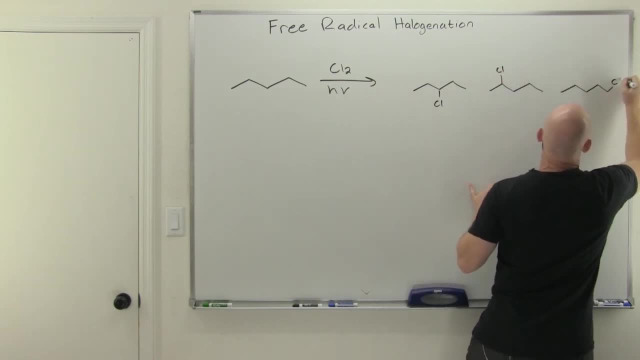 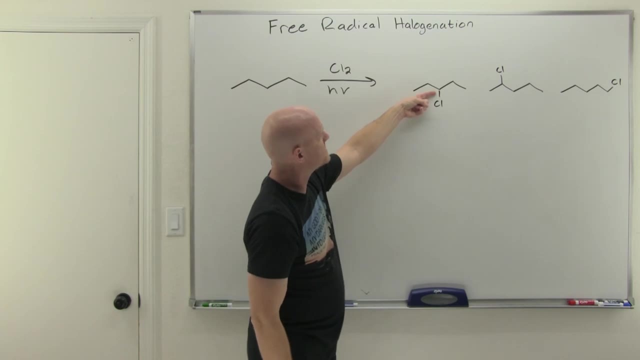 on one of these or finally on one of the end carbons- and these are my options, and if we're including different stereoisomers. we then got to go back and say: did we form any chiral centers? well, when we substituted for a hydrogen here with this chlorine, that did not turn into a chiral. 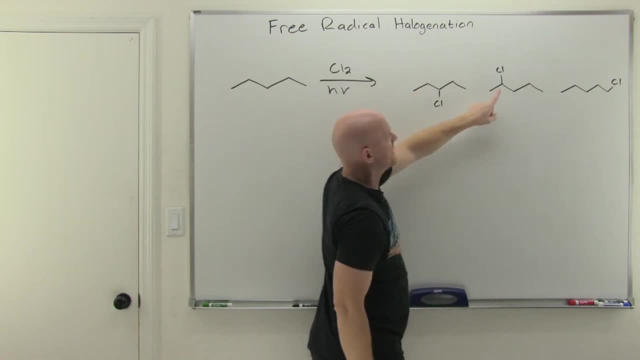 center. it doesn't have four different groups because it's got two identical ethyl groups. but on this one, that is indeed a chiral center, it's got four different groups and you can, in principle, if you replace one of the hydrons, you'll get r, and if you replace the other one, you get s and you're. 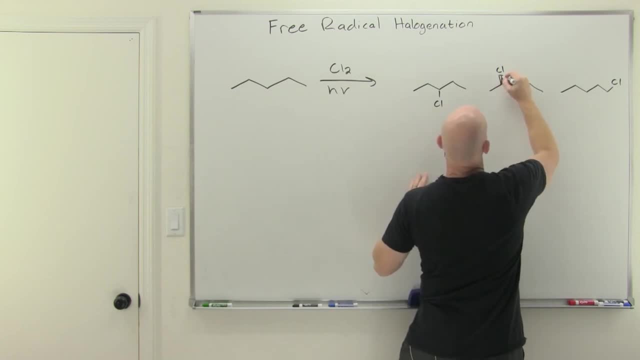 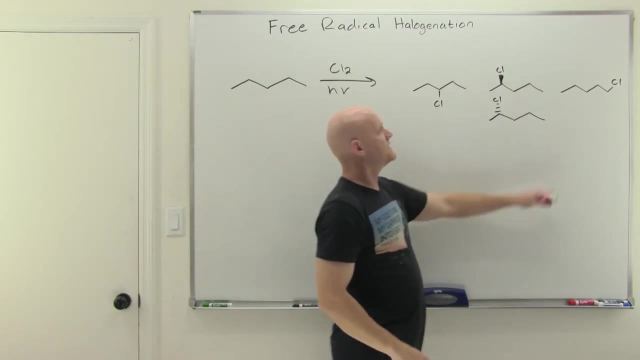 going to get both, and so in this case, we're going to take the time to draw both, since we were told to include all the different stereo isomers. all right, so there's two. and then, finally, we've got this one here and where we substituted for the chlorine there, it is not a chiral center, so 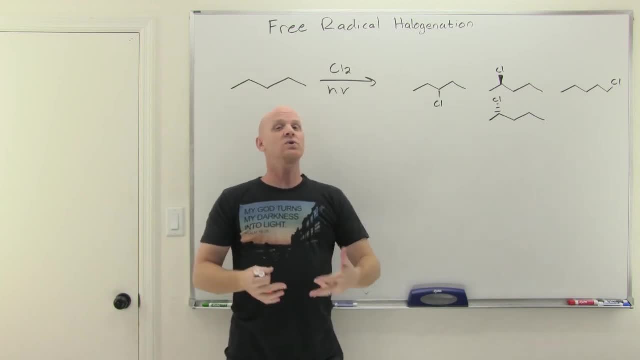 only one version of that molecule and in the end, as long as we're including stereoisomers, we would get four different monochlorination products doing substitution just once with a chlorine. now if it said exclude some of the monochloric products, we would get a chlorine and then we would get the